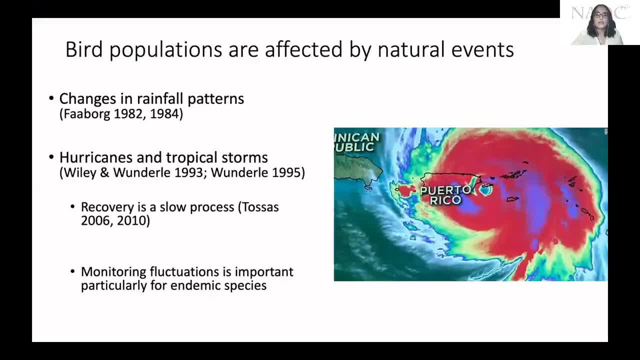 My name is Adrienne Tossos, I am from Puerto Rico and I work at Birth Caribbean. I have a PhD of health and social care at the University of Puerto Rico and I need to ask you what is your opinion on persons who have tired, who are sick or who are in dire need of help. Dr Adrienne Tossos is the first presenter and I will be the first presenter. What are some of the factors that have affected birth? Dr Adrienne Tossos is the first presenter. My title is Dr Adrienne Tossos. I am a mommy, τη, and I am a caring mom. 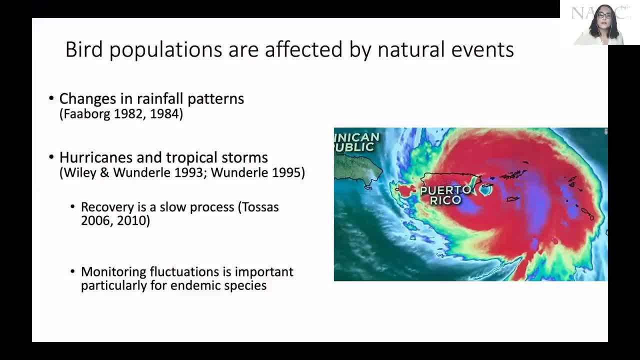 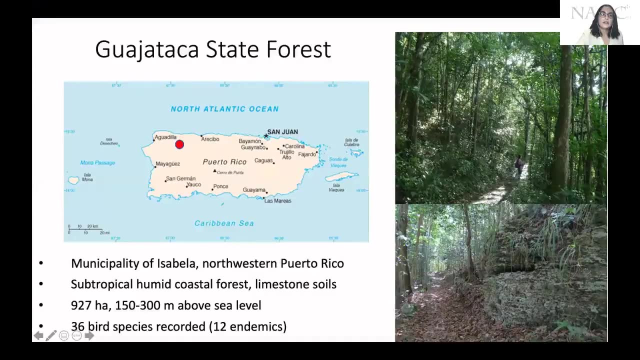 when there were no natural events going on, but it's important to know what is the status of endemic bird species. The work that I've been doing is in Oaxaca State Forest, As you can see here in the red dot. in the northwestern part of the island, the Oaxaca State Forest is typical. 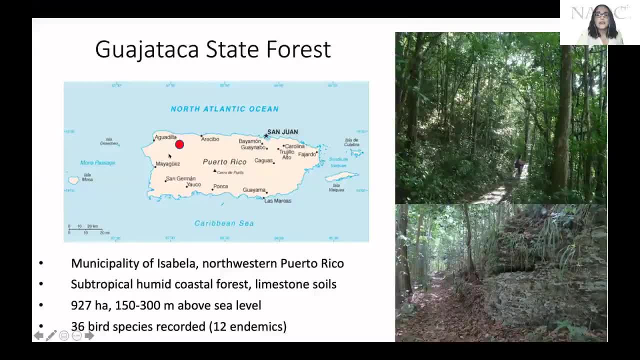 of the subtropical humid coastal forest. It lies in the north coast of limestone soils. This is a small forest of 927 hectares, 150 to 300 meters above sea level. We have recorded 36 bird species and 12 of the island's 17 endemics. 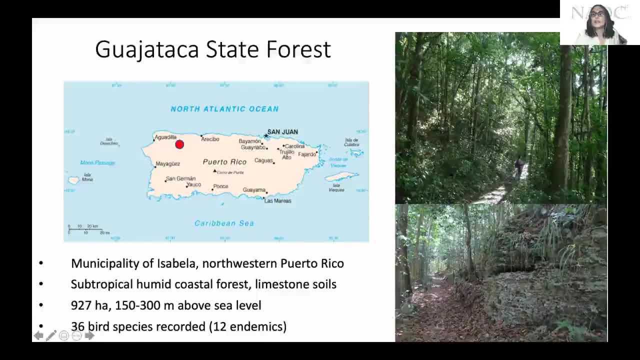 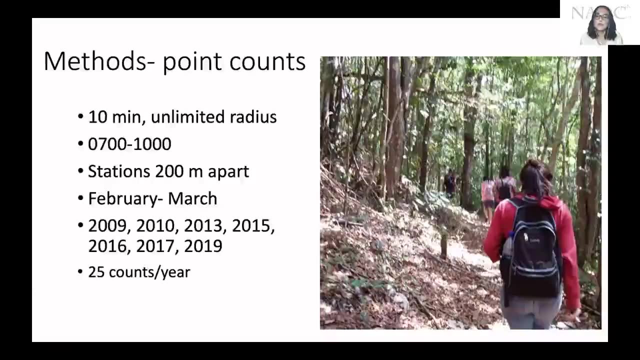 As you can see in the pictures, normally the forest you can see with a closed canopy is a closed forest and you can see this: the limestone soils. During this decade-long project we have done point counts in different trails. I selected a subset of plots of point counts for this analysis, All the point counts that I'm presenting. 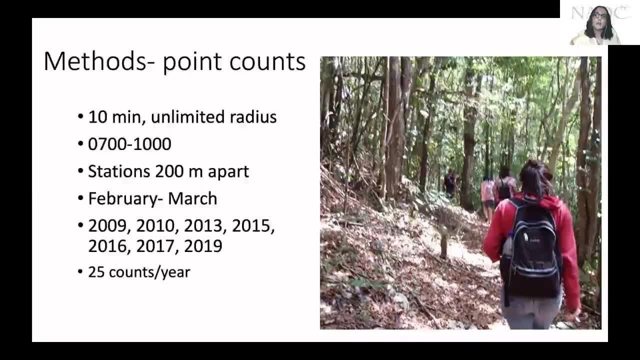 here were done in spring sessions of the different years from February to March Almost. every year. there is a point count for each of the different years from February to March Almost. every year in this decade, starting in 2009,, 2010,, we have data from 2013,, 15,, 16,, 17, and 19.. All point counts. 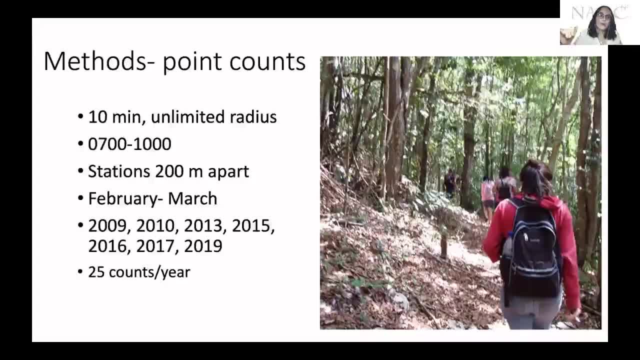 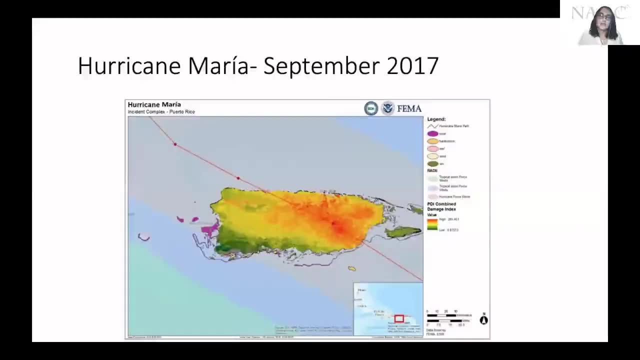 consisted of 10-minute counts recording all species heard or seen in an unlimited radius, done in the mornings, and all stations were 200 meters apart. Most of these years didn't occur in any natural event. that was of significant importance since the beginning of the study in. 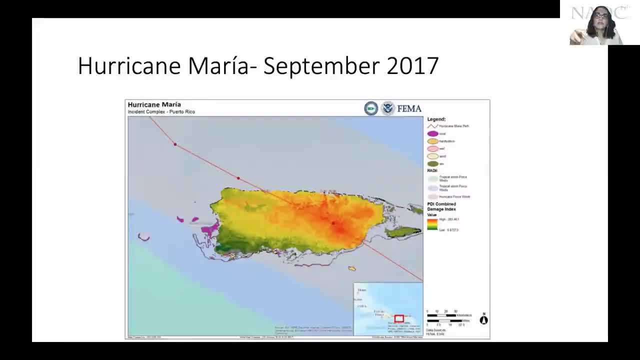 2009,. but, as we all know, this Hurricane Maria, which was a Category 4 when it crossed the island, hit hard all the island when it crossed, entering the island from the eastern coast and crossing diagonally and coming out from the northwestern part of the island particularly. 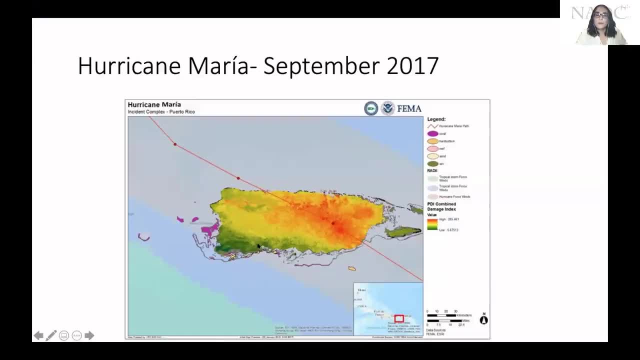 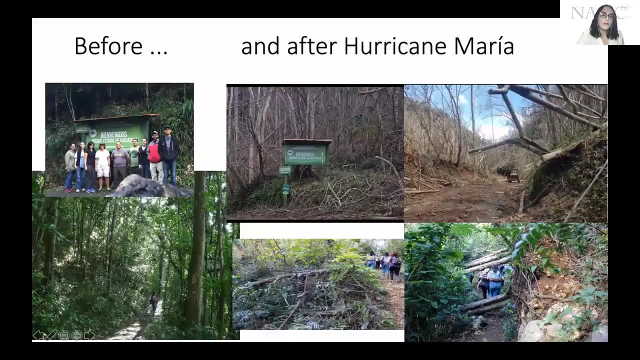 in the northern part of the island. This is a picture from the study site. We can see in the left pictures from the years before the hurricane, as seen before the closed canopy and you can see a group picture of the students. but right after the hurricane we can see the strong. 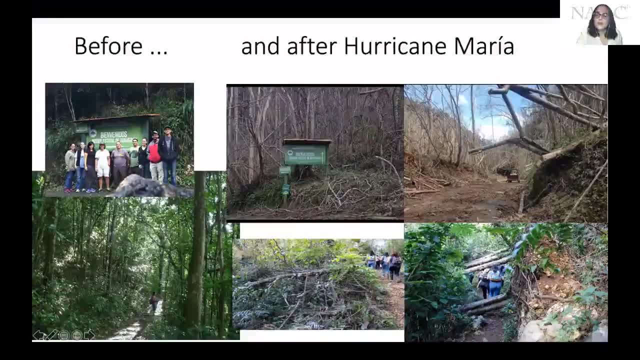 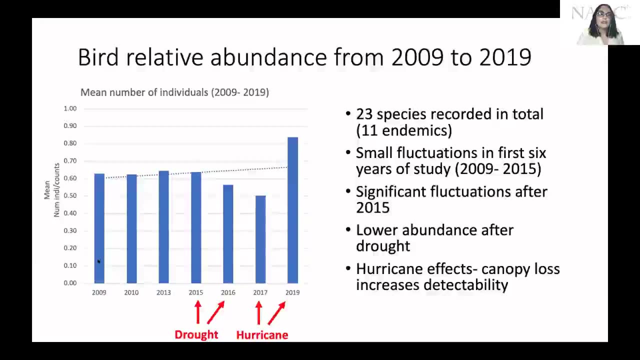 effects of defoliation, uprootings, falling trees and tree branches breaking, and one of these pictures shows the same place as before. You can see the drastic effects caused by the hurricane When I analyzed the data for this decade, starting in 2009,, there are small fluctuations in the first 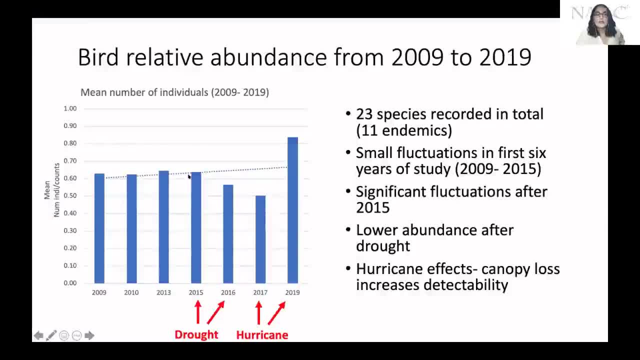 six years, but nothing that is very impressive. but then we had this change drastically after 2015,. we can see a drop in the data in 2016, and this is the year of the hurricane 2017.. What we know? the effects of the hurricane, but I wasn't counting on finding this decrease. 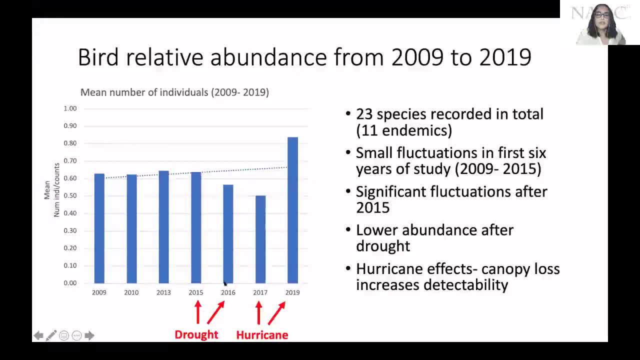 in the relative abundance of birds in 2016,, which was very evident, but it was caused by a drought, so the forest stayed the same, but we could see an effect dropping in almost 20% of the populations of the birds and the effect of the drought. 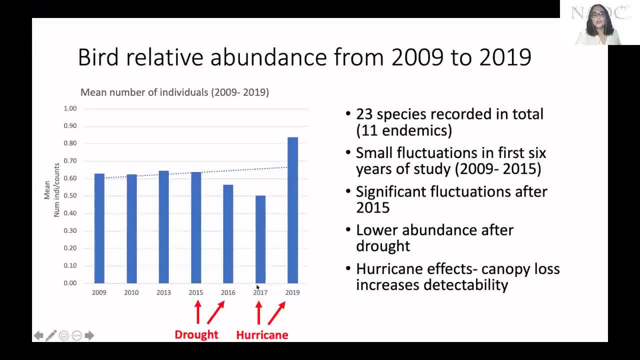 lasted for two years, so it was a long-term effect. When I see the data from the 2017 year, when the hurricane passed through the study site, the effect is very different because, instead of seeing a decrease in the relative abundance of birds, I can see a higher number of bird. 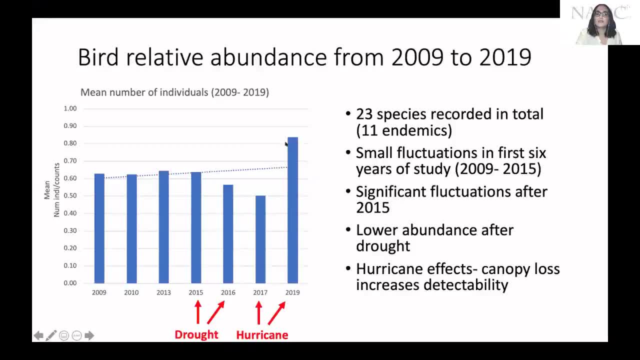 counted, but this is an effect of the loss of canopy. when you're doing point counts, You have not many branches, not many leaves, so you detect more birds and this is the effect of a hurricane. In this point counts we found 23 species. 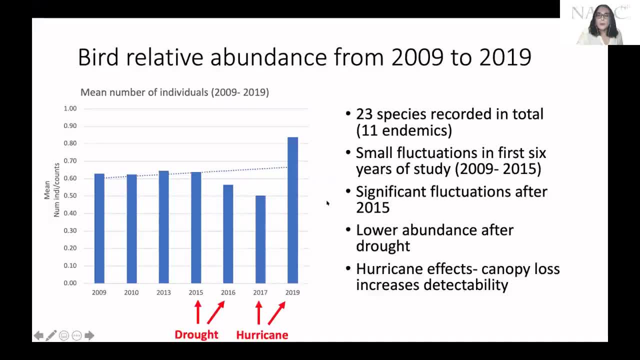 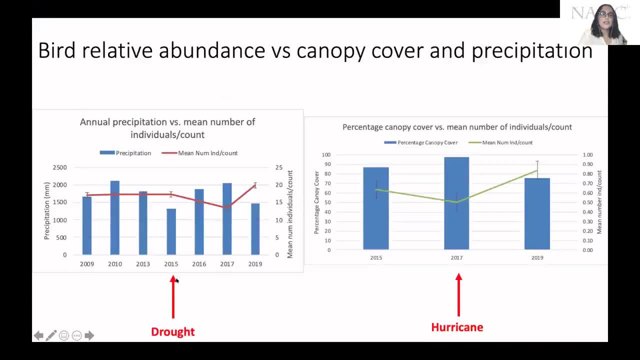 recorded 11 of endemics. When I compare this with the precipitation data, I can see here the bars showing the precipitation in millimeters. This is the drought year 2015.. It was a severe drought, with less amount of rainfall than the previous years, and when you see the line of the number of birds, 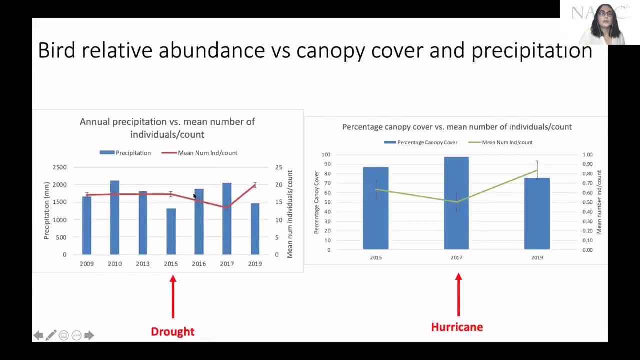 recorded not that year, but the two years after the drought. you see drops in the number of birds that were recorded And the number of birds started to increase after the hurricane- I'm sorry, after 2017, but this is the year that the hurricane crossed the island. So here is. 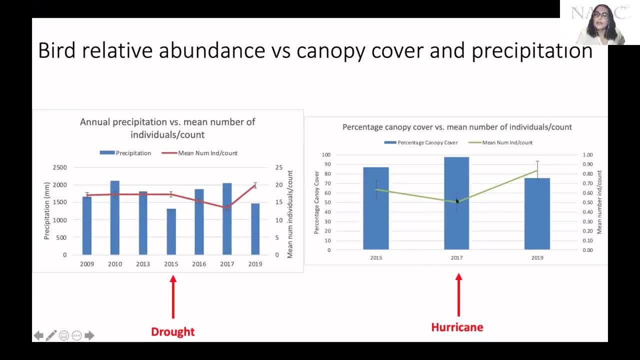 in the right, another graph showing the relative abundance of birds compared with the canopy cover and the bars. the blue bars are showing the canopy decrease significantly after 2017.. And the number of birds increased but, as I said before, the increase is due to the 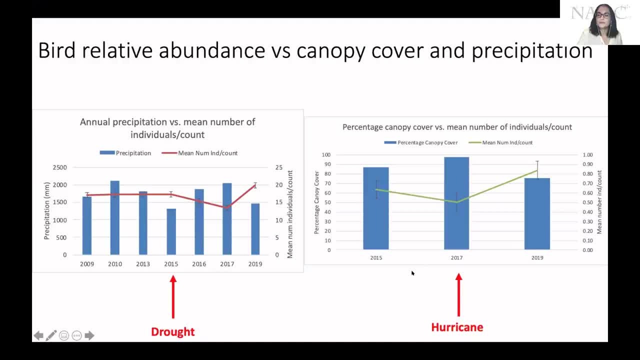 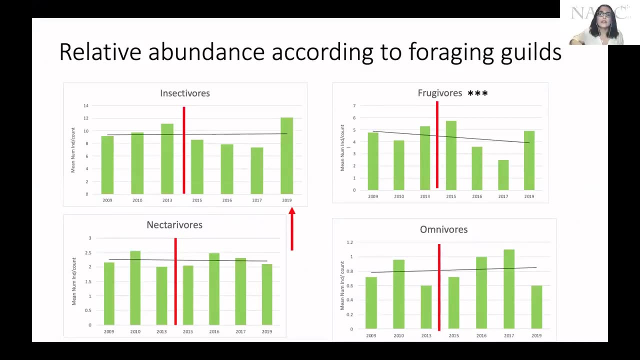 higher detectability. This same effect was found by Wunderli after the hurricane Hugo in the Junque Forest. When I evaluated the data according to the foraging yields, I have a red bar separating the buildings. I think it's even more the first part of the study, the first six years, with small fluctuations, but no. 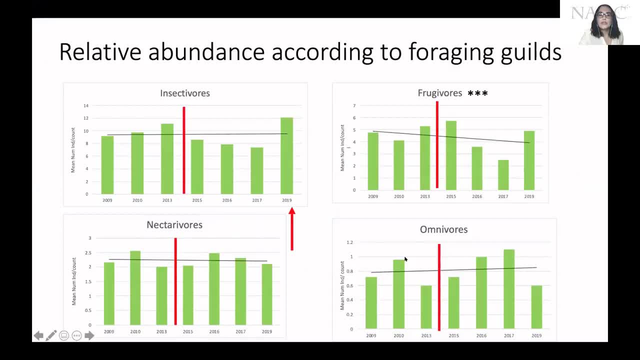 significant changes for insectivores, frugivores, nectarivores and omnivores, But I can see here an increase in insectivores after the hurricane. This foraging guild, apparently, is the one that benefits more from the restoration of the forest after a hurricane, with new leaves probably more. 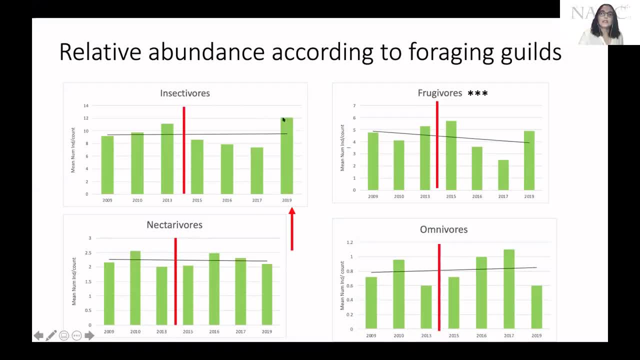 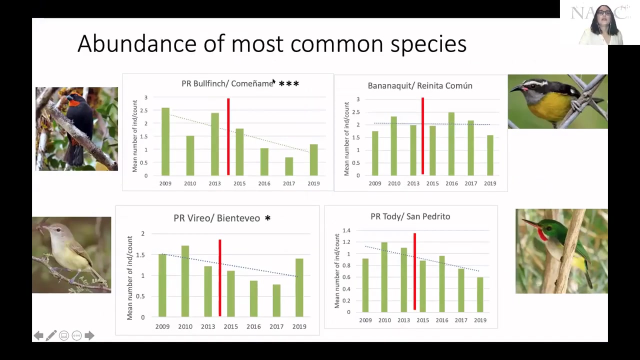 herbivore insects, so insectivores benefit from that, But the only foraging guild that changed significantly was that of the frugivores. This was the birds that changed more drastically. When evaluating the data for species individually, there were some. 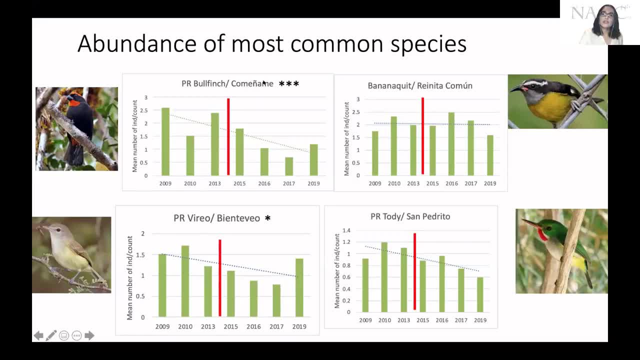 significant changes. There was a significant difference for some of the species, not for others. For instance, the banana queen is a very common species and did a flu-to-eight much before or after the hurricanes, or before and after the drought, but the Puerto Rican 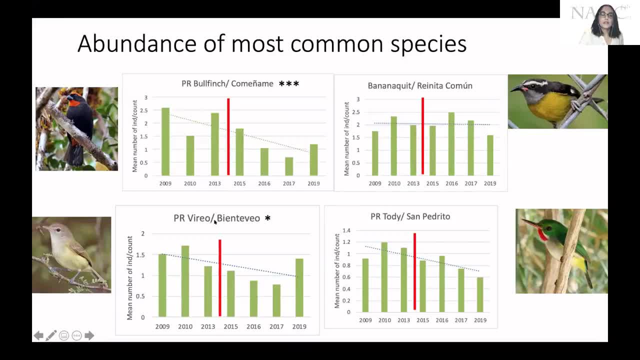 bullfinch, which is an endemic, decreased significantly. The Puerto Rican birrio decreased significantly, But you can see that two years after the hurricane in 2019, both species are starting to increase again. Other common species in the in the forest that were 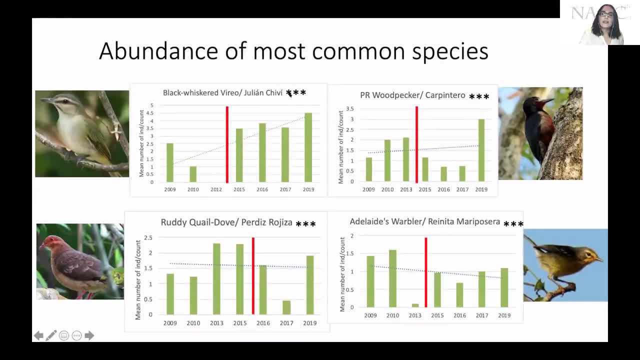 the black whisker burial was affected significantly, but these species have shown to increase also after two years after the hurricane. There are some species that had different behaviors and, for instance, the black whisker burial. we cannot see much of the species in some years, but this is something that depends. 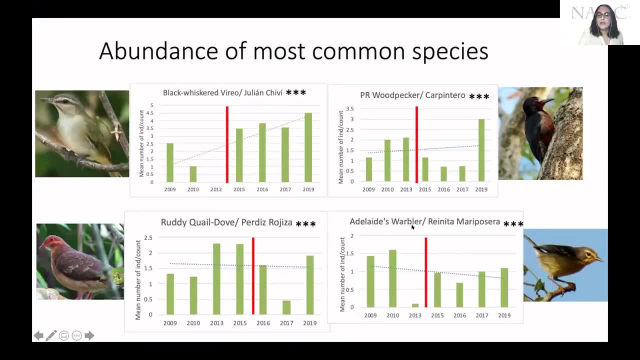 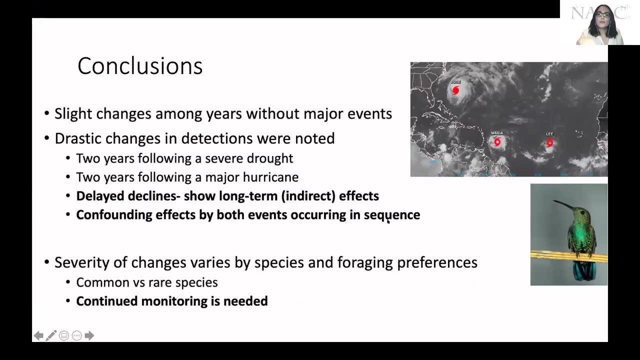 on the behavior of the species. The Adelaide warbler is some species that I need to figure out. what happened in a year where, when we didn't have records- So concluding- there were slight changes, some on years, with the duration, but there were drastic changes in detections up to two years. 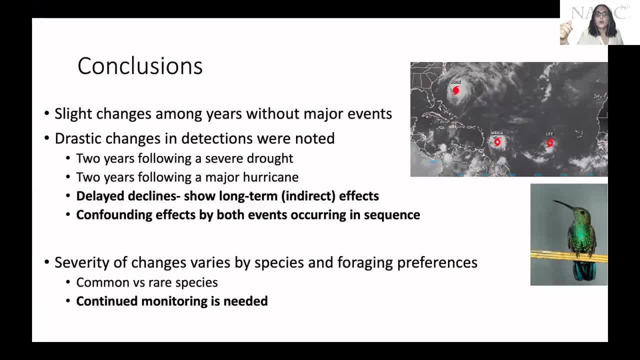 after a severe drought, There were also drastic changes two years following a hurricane. These changes were delayed because we could see that they lasted more than a year and it reflects that these are the indirect effects that natural events can cause, probably changing the micro habitat, the resources. 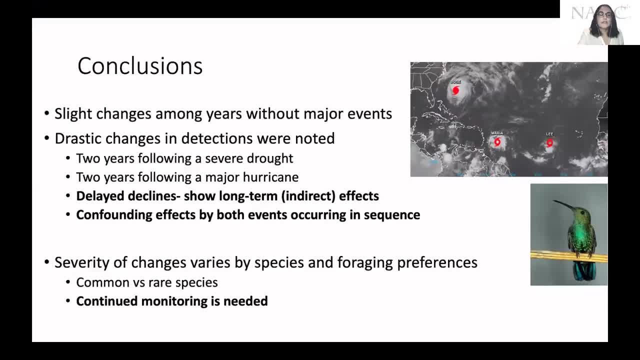 that the species need to feed and other characteristics. But what if we have both of these kind of events going on in a sequence? We saw here a drought followed by a major hurricane, But also there's a variety of changes that vary according to species and their foraging preferences, And this was not very common. 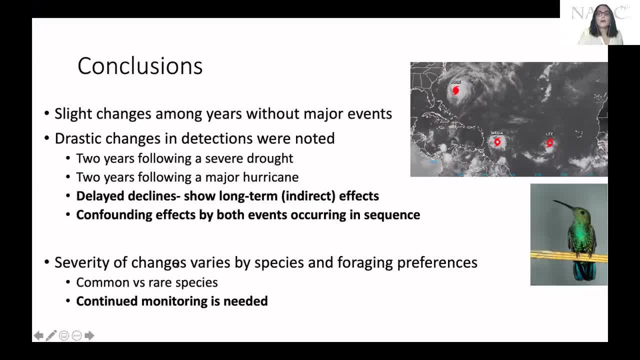 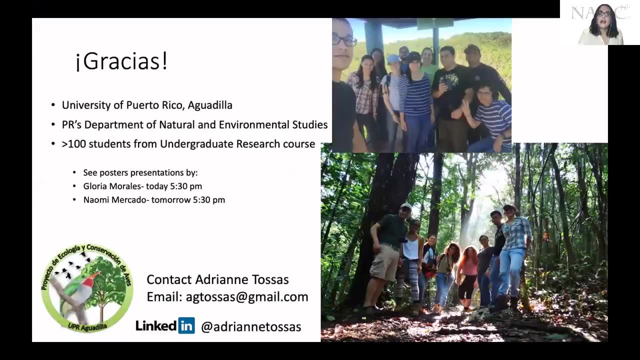 not a very big problem for common species, but what about rare species? To know what are the long-term effects, we need to continue monitoring. I want to thank my group of students. The students vary every year because each year they have a different site, So we would like to thank their 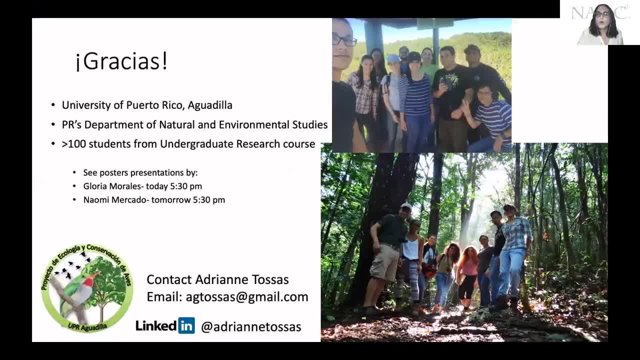 because I have been participating in this research as part of a course. So I have had more than a hundred students passing through this course for the past 10 years And it has been a great experience to have them participating. They have this experience and it helps them. 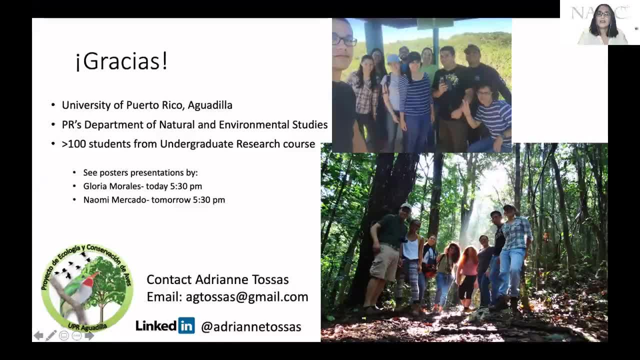 to apply for graduate programs and to prepare for their professional career. So mostly of them follow different paths like biomedical sciences, but there are some that are going to graduate school in ecology as well. I have two of my undergraduates presenting posters today and tomorrow. 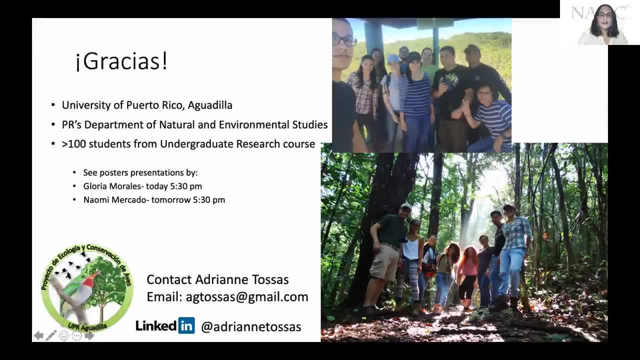 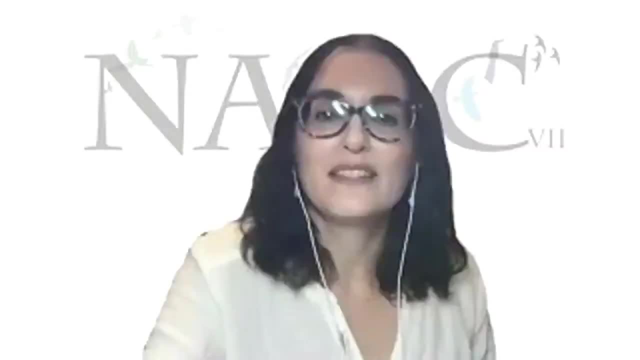 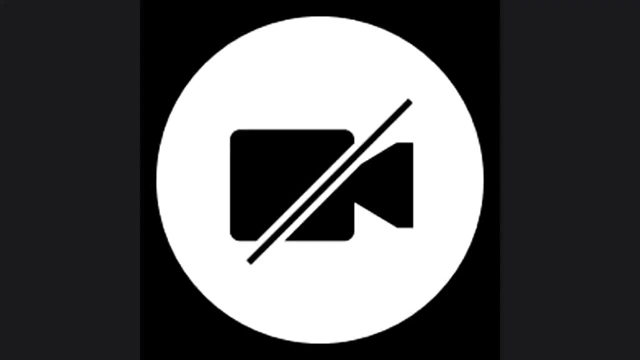 So please see their presentations And I'm here to answer any questions if someone from the audience is interested. Thank you, Adriana. there are three questions. I think we would have time maybe for one or no, Should we fit one in? 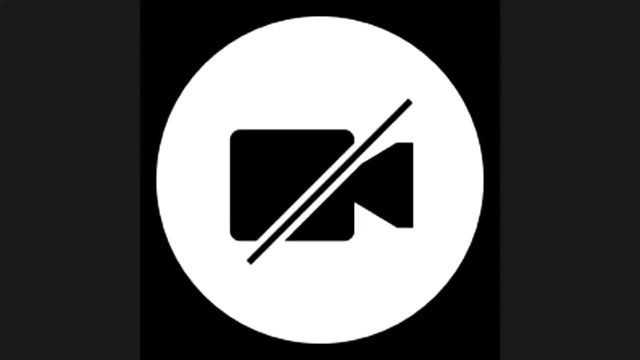 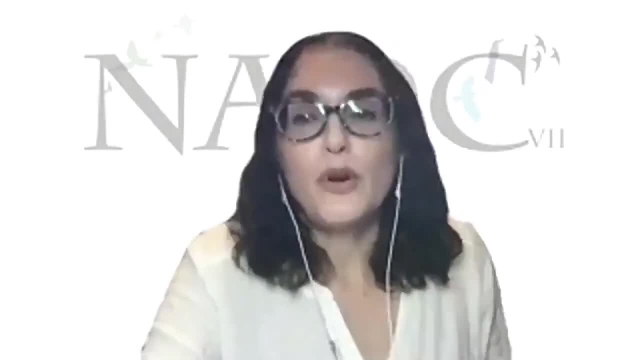 OK, we can have one Great talk. Adriana, Why do you think the Puerto Rican bullfinch was particularly badly affected by the drought? Probably because of the food resources. It's a frugivore, So the drought can cause less food available. But We have to keep monitoring. The rainfall patterns was showing a small drought in 2019 also, So we will need two or more years to know how is the population, But at least it didn't decrease to a bad level. These species have shown to bounce back. 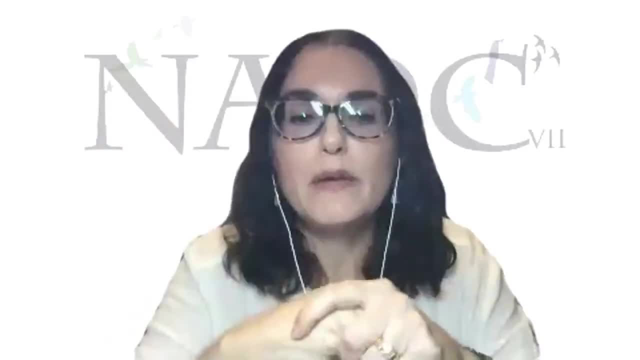 So at least the common species are not doing that bad. 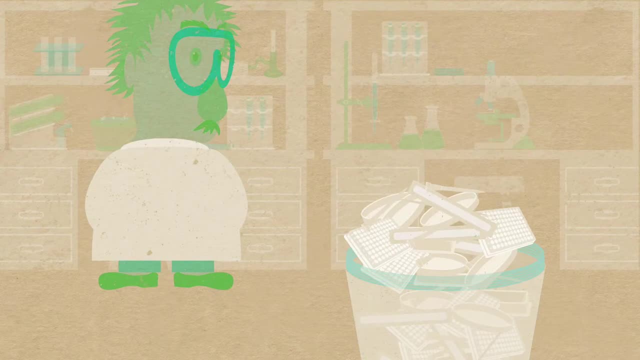 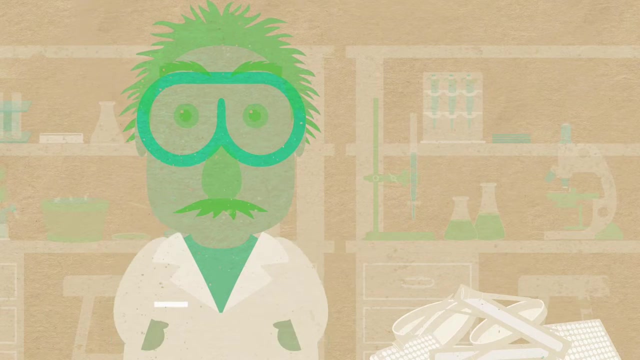 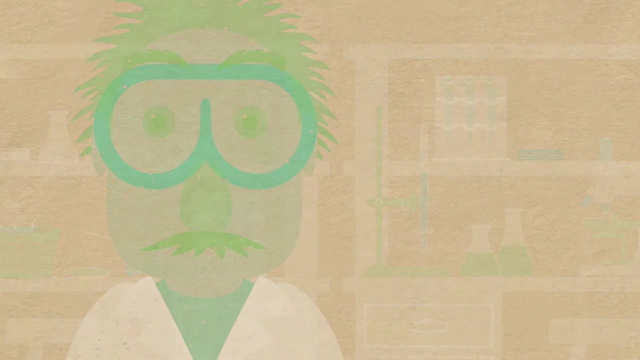 Hey you. You there in the lab coat and goggles. Have you ever stopped to think how much potential recycling a typical researcher creates over the course of a day? What about how much energy a room full of minus 80 freezers use? You're not alone. There are so many things competing for. 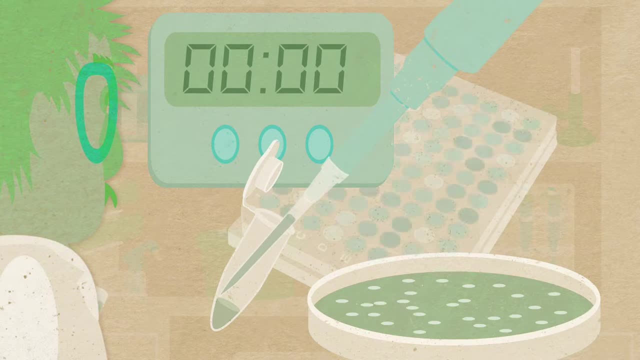 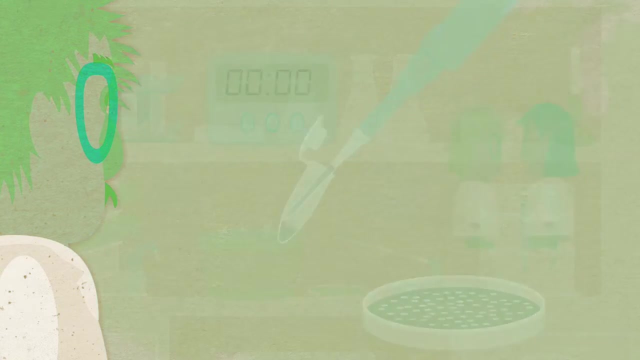 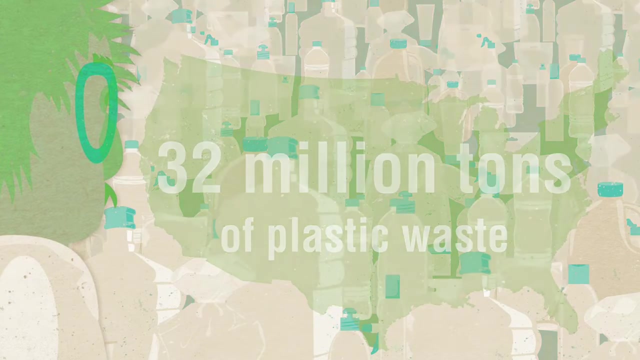 your attention when you're at the lab bench, It's easy to understand why you haven't noticed how many petri dishes or microcentrifuge tubes you've tossed out. Did you know that around 32 million tons of plastic waste were generated last year in the US alone? While we can't say for sure how? 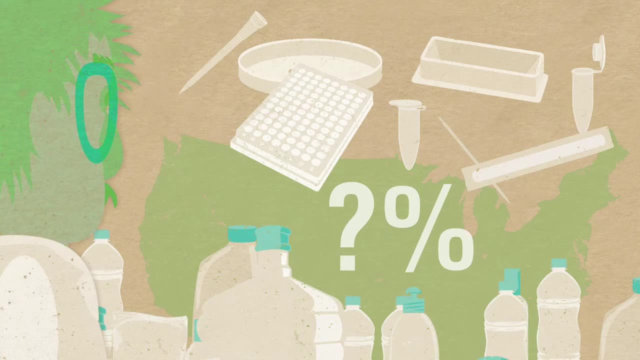 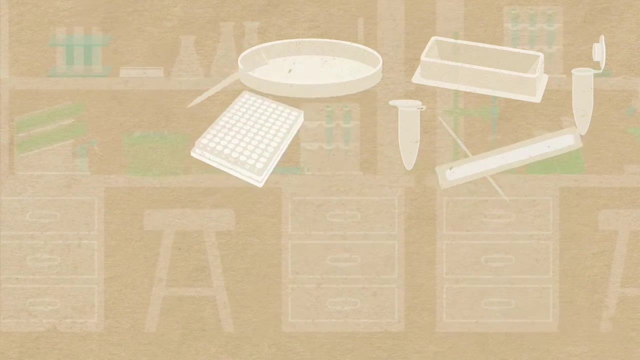 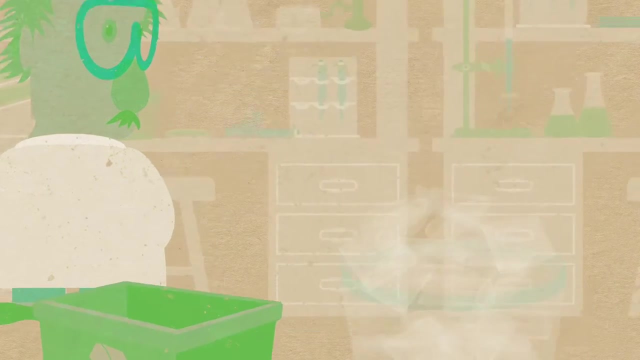 much of that was generated by life scientists engaged in research. we can say that we definitely share some of the responsibility. We know that scientists use these tools to make discoveries, cure diseases and solve problems- Mysteries- but all of these tasks create byproducts that could be recycled. 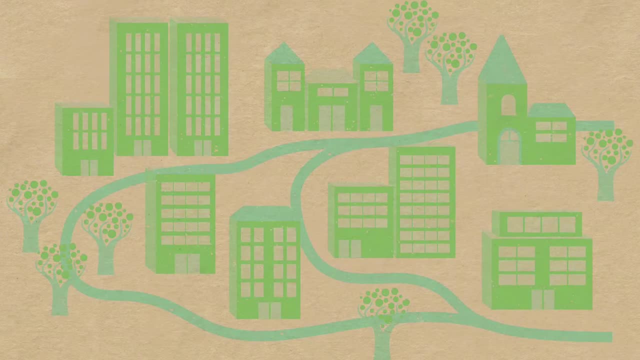 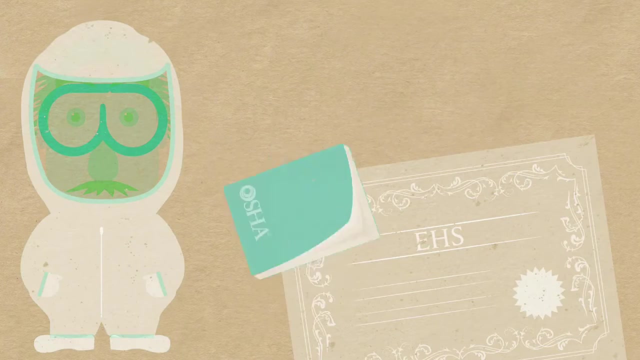 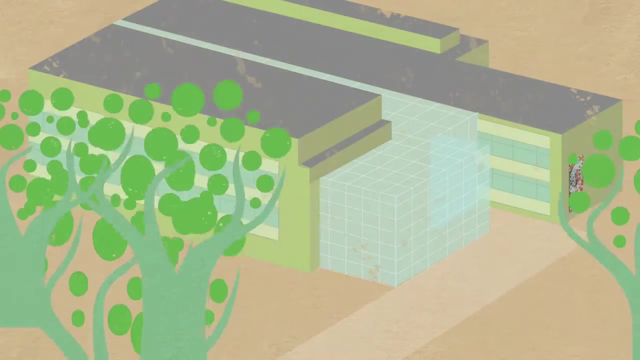 Spread over a lab, a department, a university, a city, state, country, you can see how quickly it adds up. Sure, there are some things that are out of our hands, but let's do what we can. Here at NEB, we are always looking at ways to help reduce our impact on the environment. We are proud to 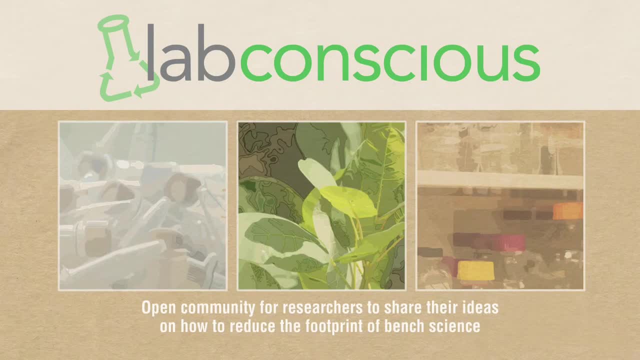 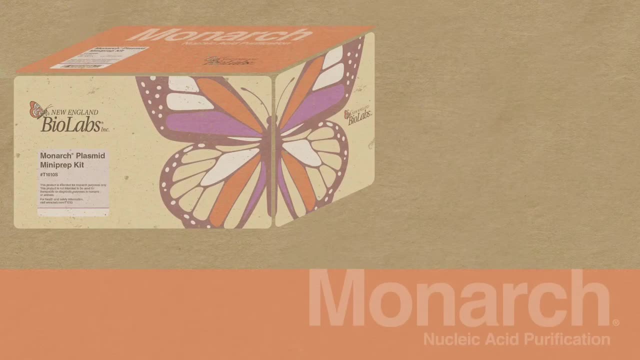 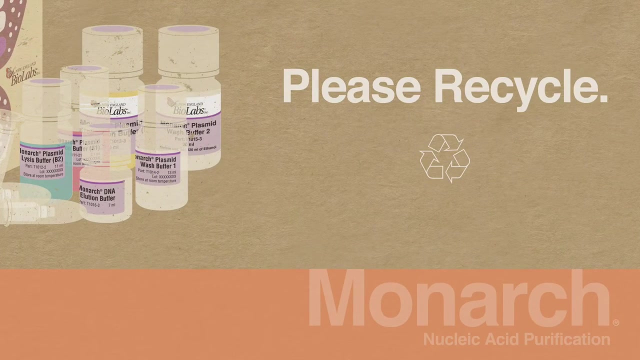 sponsor: Lab Conscious. Lab Conscious is an open community for researchers to share their ideas on how to reduce the footprint of bench science. We also carefully designed our monarch nucleic acid purification kits so that they use less plastic and are packaged using responsibly sourced, recyclable materials. We encourage you to share. 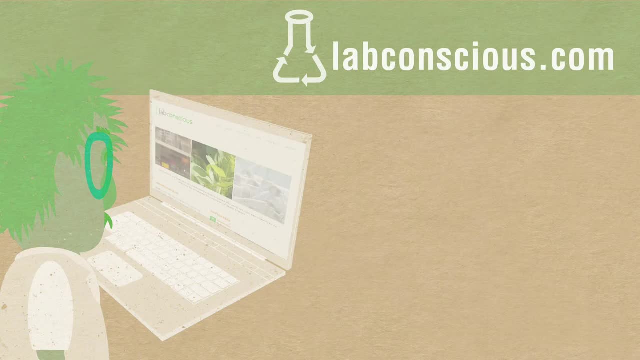 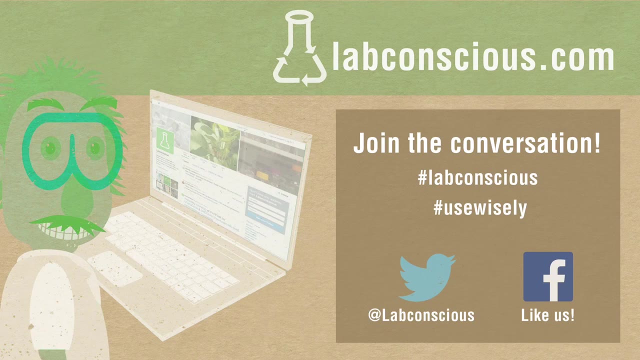 your suggestions at labconsciouscom so that we can all benefit from each other's ideas, big or small. And at NME we provide evidence that the use of NME for biochemical samples is a good practice of the scientific research we do- tripalincom. 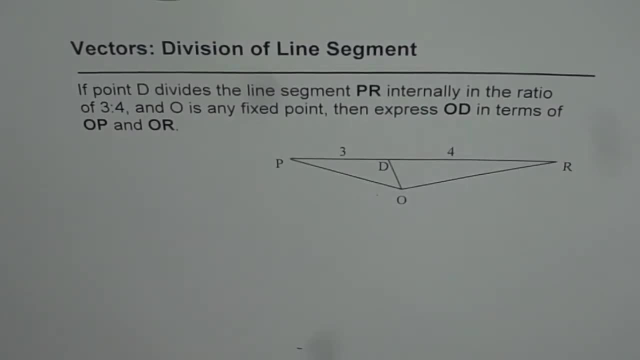 Vectors: Division of line segment. Here is an example to understand how to find the coordinates of a point which can divide a line internally. The question is if point D divides the line segment PR internally in the ratio of 3 to 4 and O, is any fixed point then express OD?